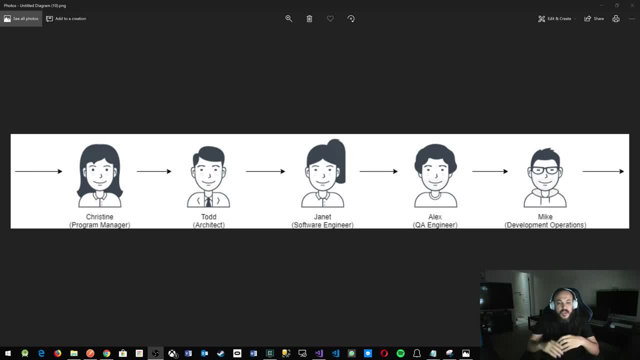 breaking that down in your Azure board into a bunch of user stories. Your architect is picking those up and designing them. She's getting those up and designing them into architecture and components that software engineers will take on to develop. Software engineers can't start without the design, The design. 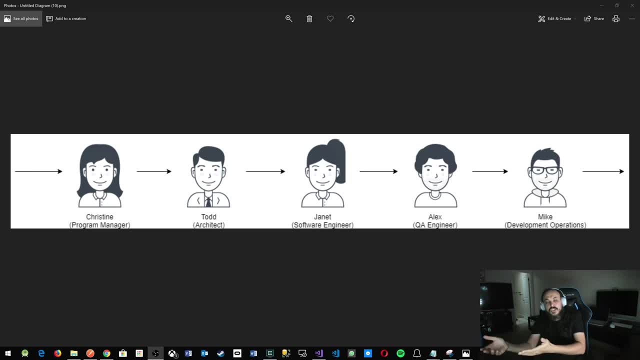 is done. Software engineers are starting to write some code, And then the quality assurance engineer can't test something that isn't developed yet, So they have to wait on the software engineers, and so on and so forth. with the DevOps right. How do we visualize and model that We? 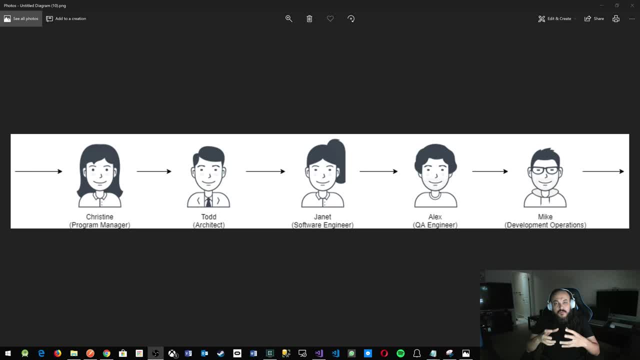 want to model that in a real world software. We want to write a program that shows us how would that look like, right? Okay, So if you look at here from at a glance, you can see that each and every one of those shares kind of two functionalities, right? The first functionality is the handling. 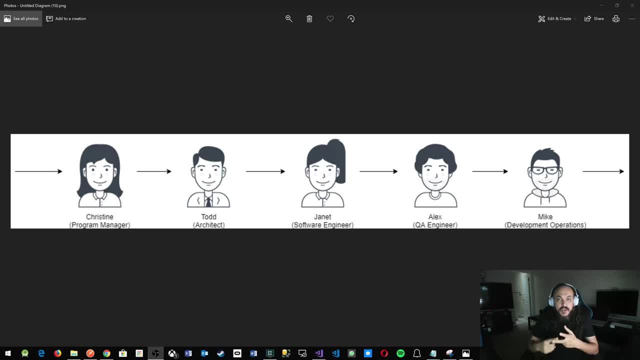 of the requirement. The second functionality is handing it over to the next person who is waiting on it to pick up on that requirement, right? So we need these two functions. so, as you thought, we're going to build an interface that dictates that both of these functions. 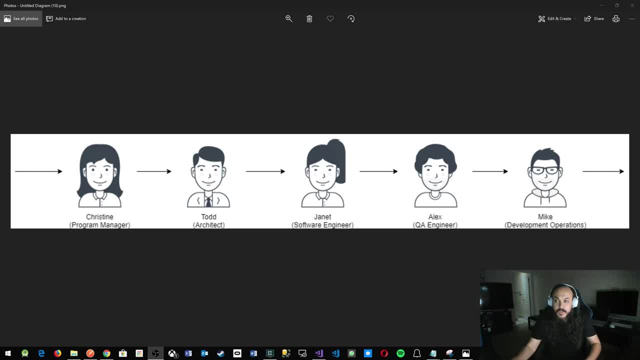 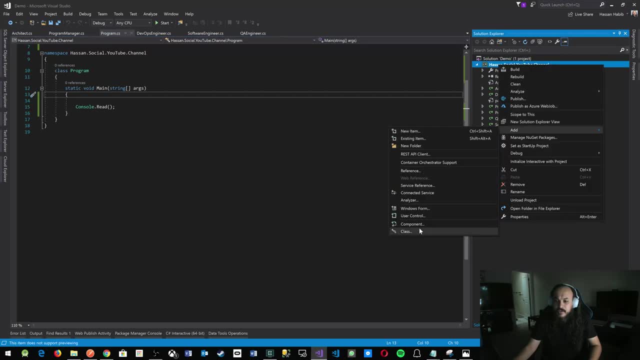 have to be there, Right, All right? Okay, All right. Let me give you a couple of photos here of these functions. they must be there. so how do we go do about that? let's go write some software and let's go build that interface first and let's call our. 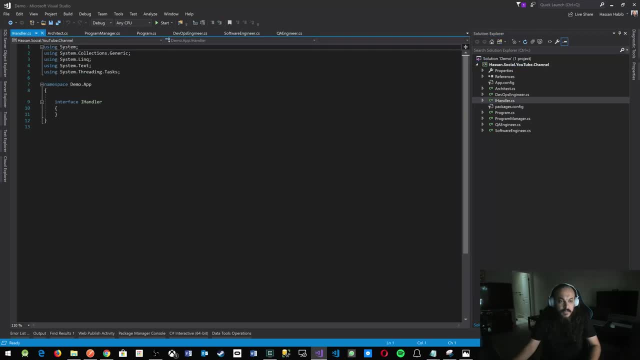 interface I handler and I handler will have a couple of methods. the first method is to handle the requirement. you're gonna build it and here a model. we can generate a quick model here. that's called the requirement. we're gonna do some stuff with it, so you're. 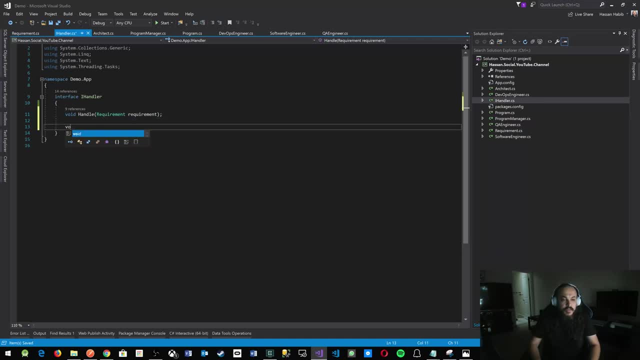 getting a requirement. you know we want to build a website or whatever. the other one is a hand hand over and requirement over and then hand handing the requirement over, you're gonna want to handle it. hand it over to someone who also implements. I handler right, so you want to hand that over after the. 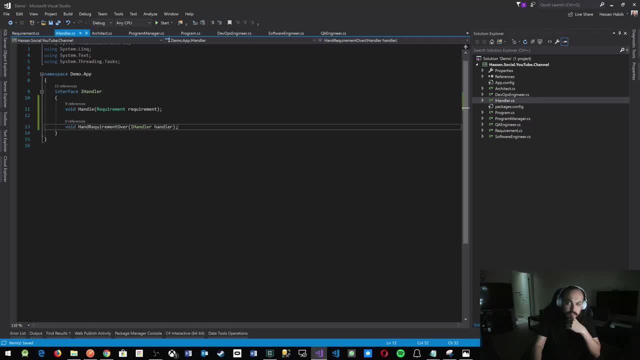 requirement is done, you know, to the next person, right and so okay, so we have these two things and then let's go ahead and fix our requirement, our requirement here. just to keep track of things, I'm gonna build a quick list in here, then I'm gonna call it operation, so we can keep. 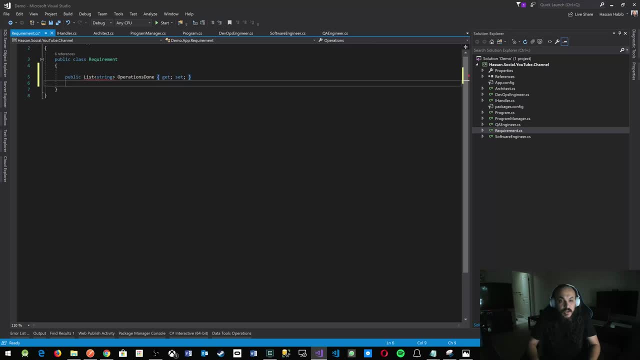 track of the operations that has been done, operations done. so when the operation is done, you know the person will go ahead and you know you know add that as an operation. right, we also need a constructor in here. so the thing is doesn't blow up. we gotta go and say: operations done, just instantiated with. 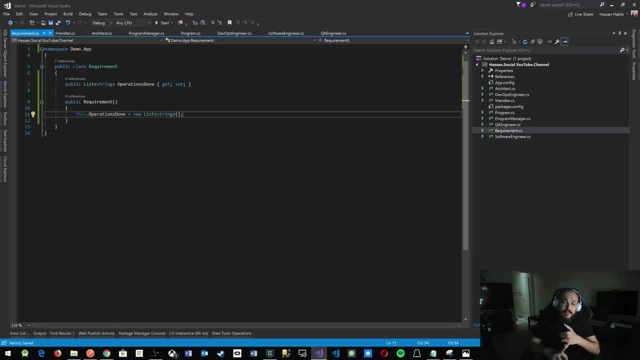 an empty list as soon as you get the requirement. all right, we have the requirement and we have the main idea. right, so we have I handler. for the time of this video. I already built something like that. I think I guess I called it hand over when done so let's just change that real quick. call it hand over when. 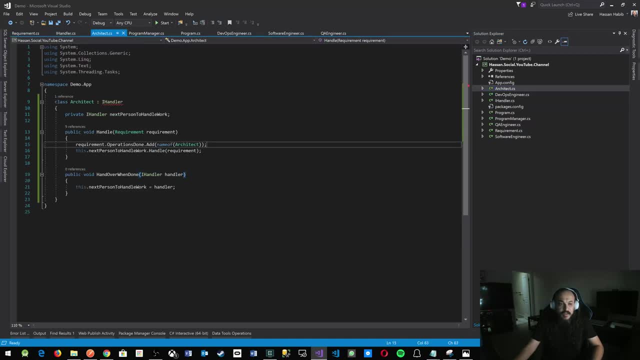 done, there you go and now everything is satisfied. so what did I do here? you know, let me what I what I did here. I did a little bit of a quick look at the information that I have here. so what I did here is that for the handle function. 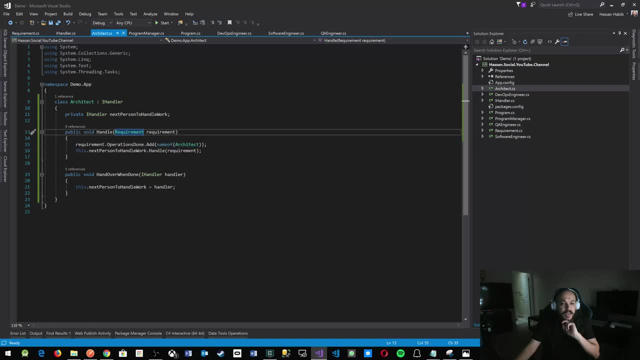 I added the operation with the name of the person that's handling this function right, and then I handed that over to the next handler. that'll take care of that requirement right. so I know the architect knows they're gonna need to talk to a software engineer after they're done, so once their work is done. 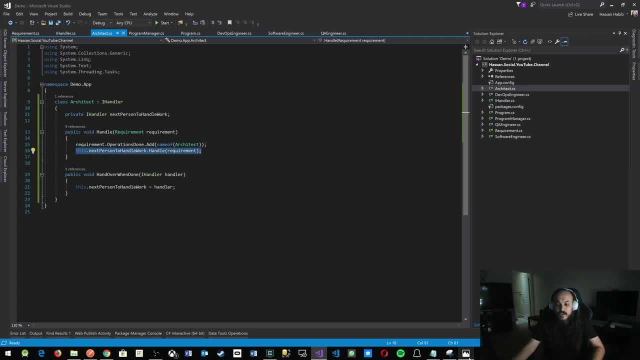 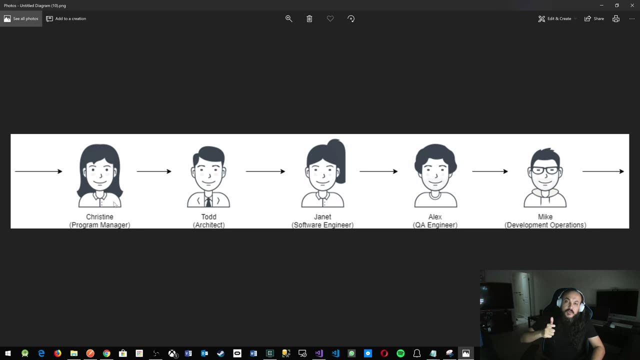 they're gonna hand that over to that person. the tricky part here is from a customer perspective. the customer doesn't see anybody except for Christine, right? so Christine will be the one that triggerer of all of that, to be the one that when she starts handling the, the, the customer doesn't have to go to Todd and say: handle and go to Janice. 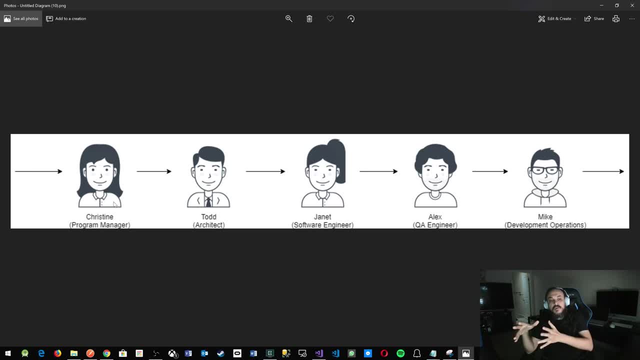 a handle, say to Alex, say, and it doesn't have to go to all these people, they just have to talk to Christine. so by saying Christine, handle that requirement, that means every single week, in every single action that's gonna follow, that should be triggered by the original handling from Christine side, right? so how does 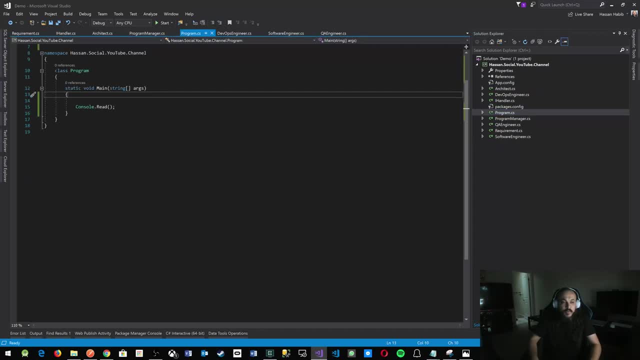 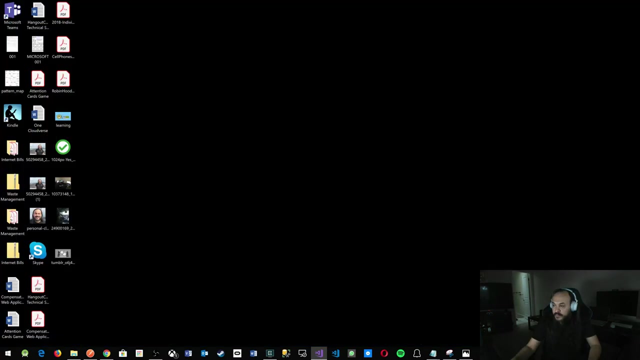 that work. let's go to the program in here and let's build that. let's build a requirement, requirement right, and then let's build the team. so I'm starting with Christine to the program manager go and then let's start with Todd, the architect, and then let me put in here the rest of the team real quick. so for 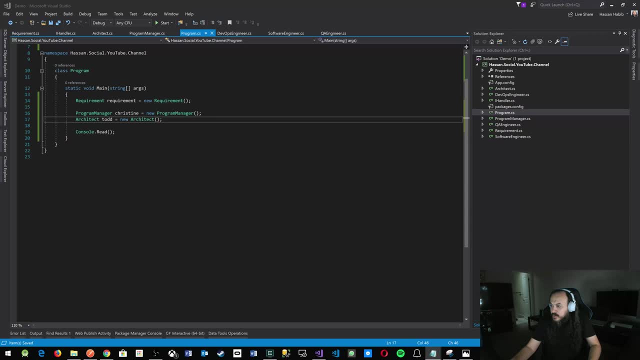 the time of this video. so here's the rest of the team. so we're recruiting the team, here's the rest of the team for you. so we're building those folk and then we're telling: we're educating these people, the folks who are to talk to. so introduce the team each other. so what? 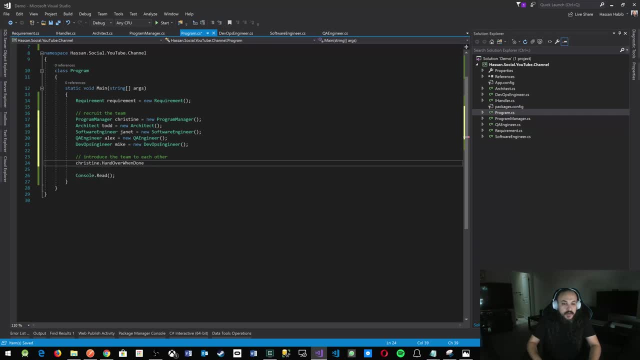 I'm gonna go here and say: Christine, please, when you are done, hand it over to Todd, and Todd will hand over to Janet, the software engineer, and Janet will hand over to to Alex and Alex will hand over to Mike, which is the DevOps engineer. something tricky here for you at. 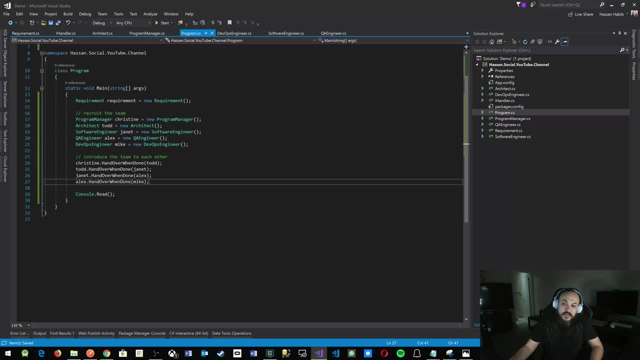 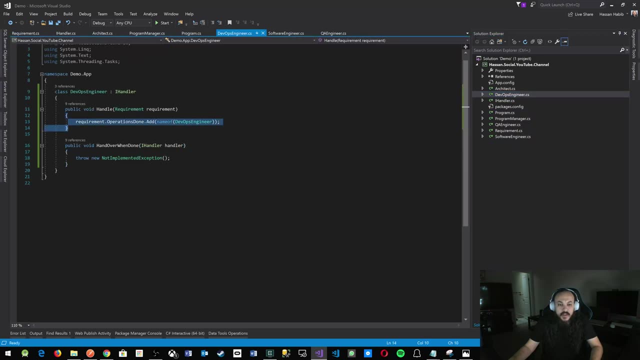 to notice. Mike doesn't need to handover to anybody. so if you go to the DevOps engineer- what I basically did in here- Mike will start calling all developers and we will see how that's gonna get right. there's handover window is not done, it's just not implemented because 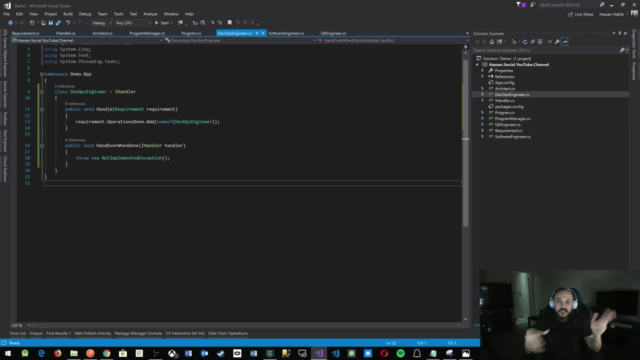 there's no handing over to anybody, right? if anything, it will just go back to Janet and then order the client right. alright, let's see if that actually works. so we what I'm going go does this test that for each VAR event in Mitch from Jeff Ryan humluty, and we would be very happy if. then, or the client, right, alright, let's see if that actually works. so we, what I'm gonna do here test. let's test that. so, for each VAR, is that trying to install? and let's just back to from Judith- is it going to workじゃ of uva. and then, and I have to, 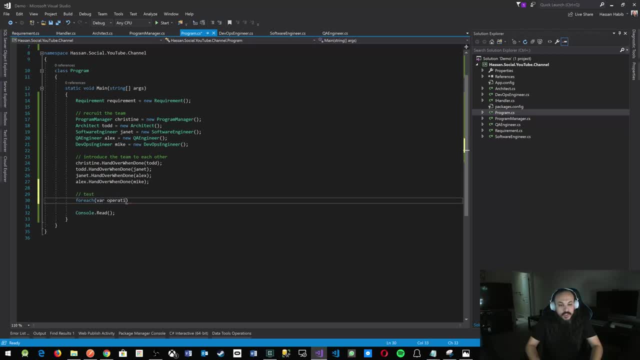 come over to the Devnya, and that's when there's on device Kennedy and there's no. So for each var operation in the requirement that operation is done, let's print out: the ideal world here is that each and every one of those should leave their mark on the requirement. 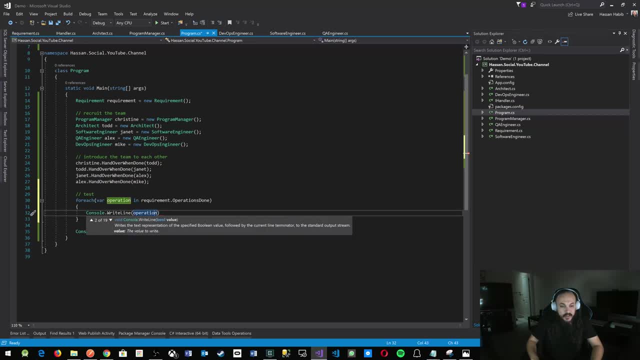 So I'm printing out the operation And let's say the operation is done, So this operation that we're printing done Now, if I run this right now, nothing happens. Why nothing happens? Because nobody talked to Christine yet, right? 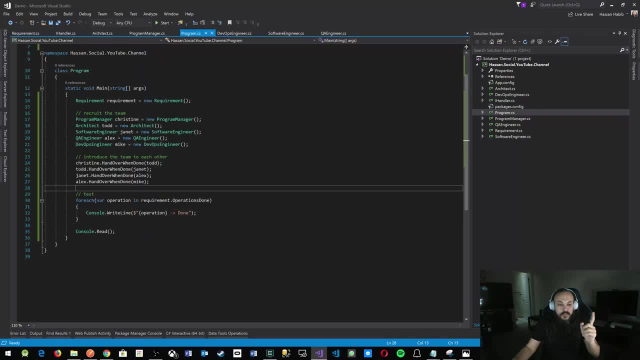 Nothing has triggered. We need to go talk to the one person that the client can see right. So let's go here and say: meet the client, Program manager. Client and program manager got together and they handed over the requirement. So Christine will say: 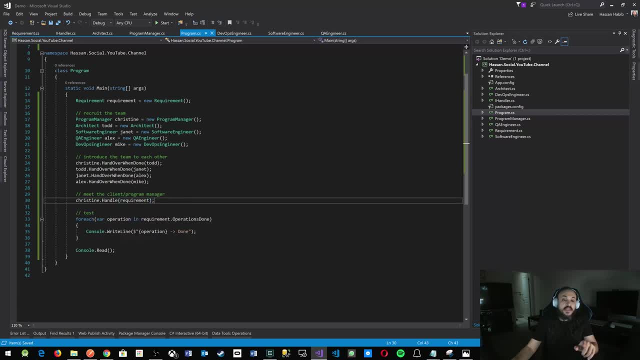 handle the requirement. That's the only thing in here that will trigger all these operations for the rest of the team. Now things have changed. If I run my program now, what we expect is that all these operations are done. So the program manager got it done. 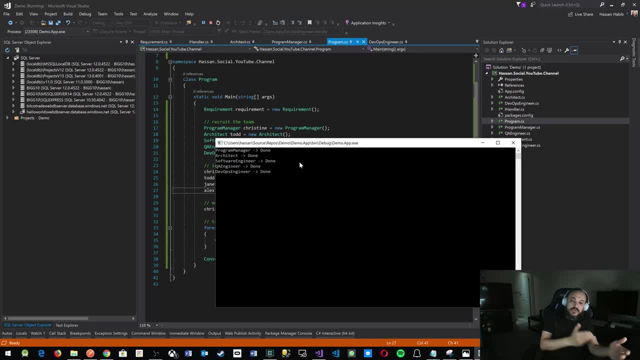 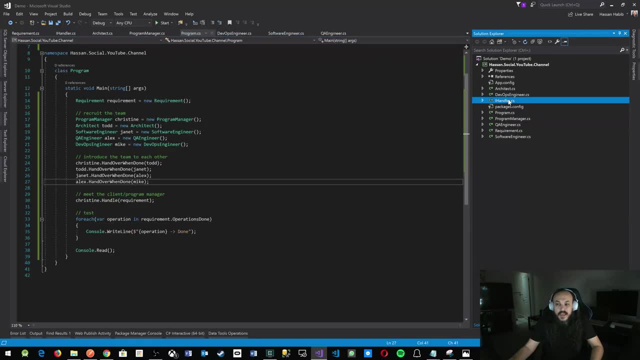 Architect got it done, Hand over to the engineer, Quality assurance and then DevOps. So you see how this chain of responsibility work. You build a bunch of classes that have to adhere adhere to certain rules based on the interface, and then you make sure each 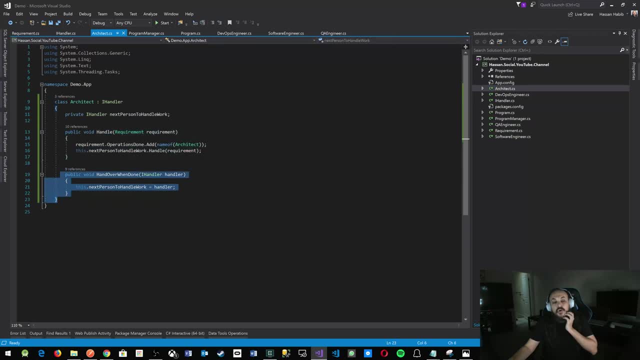 and every one of those is doing the handling and the handing over right Now. from an academic standpoint, there is different terms that people may use when they're speaking about this pattern from an abstract standpoint. right, I want you to visualize the pattern, understand what things do, rather than 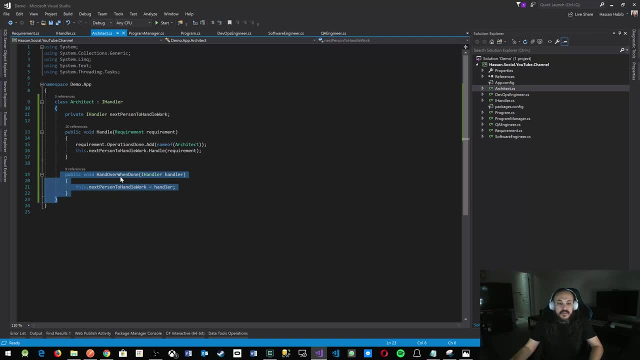 memorizing some terms right. So whether they call it a pattern, whether they call it a pattern, whether they call it a pattern, whether they call this: you know sit successor, or you know attach successor, or whatever the handling they would call it, that doesn't matter. 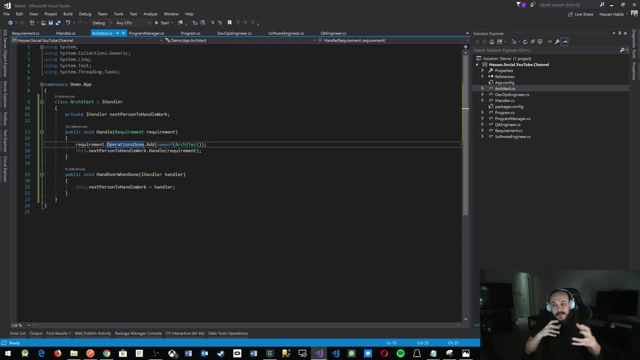 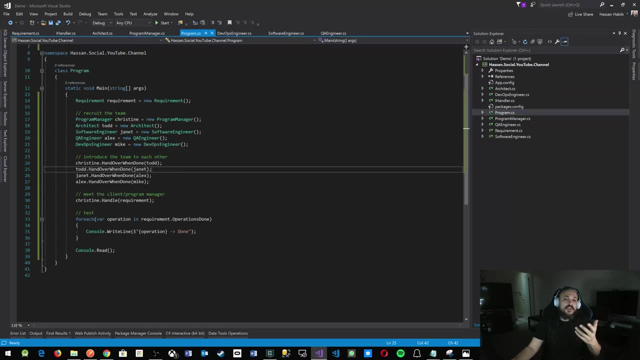 You have the pattern, You understand how it works and then you could use that. There are some drawbacks for this pattern. while we're talking about it, It's very stateful Like, for instance, what if the architect failed to finish the design? 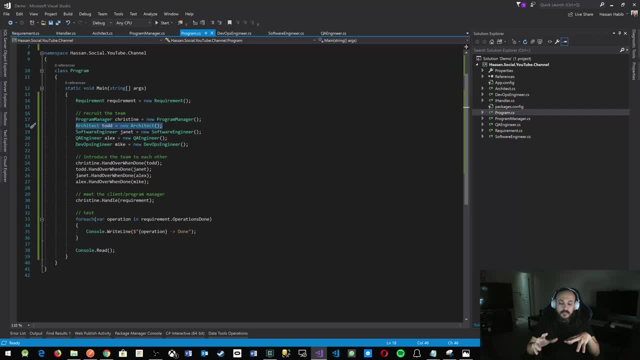 Now everything crumbles right. Now you need to do to have some mechanism to roll back the stuff that happened to that requirement up until this point. We need to roll back all the work so you don't have some bad data stuck in your database. 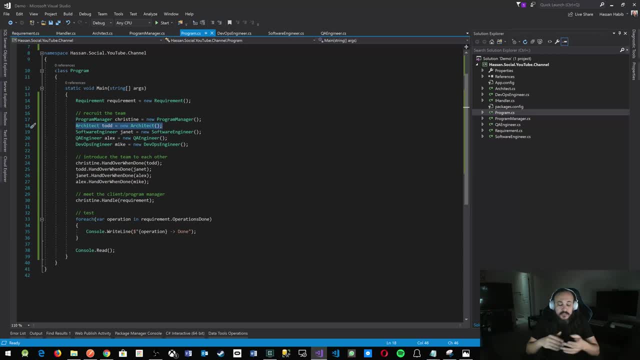 about some requirement that was never done. You may think about the memento pattern that I talked to you about before. In the real real world it's very unlikely to find a pattern like this. You'll come across software that does implement that pattern, but in today's 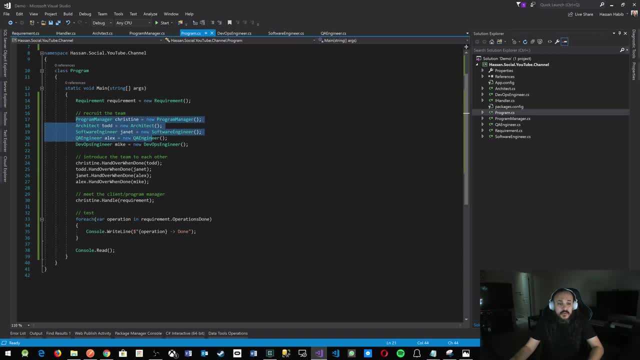 world. people think about each and every one of those as its own microservice or lambda, And when the microservice is done it goes and calls the broker class and it goes and calls the next microservice and the next microservice. It's very stateless, right.